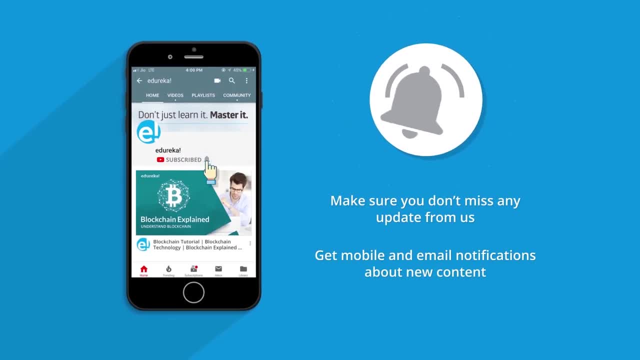 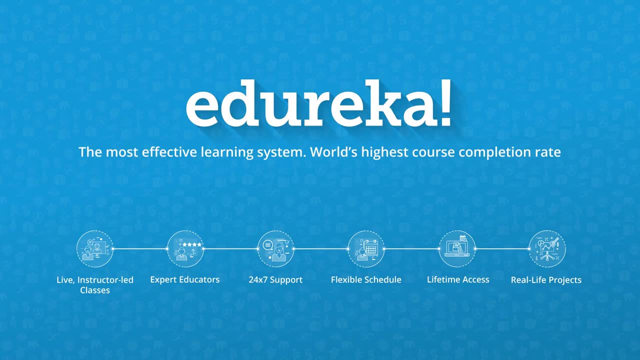 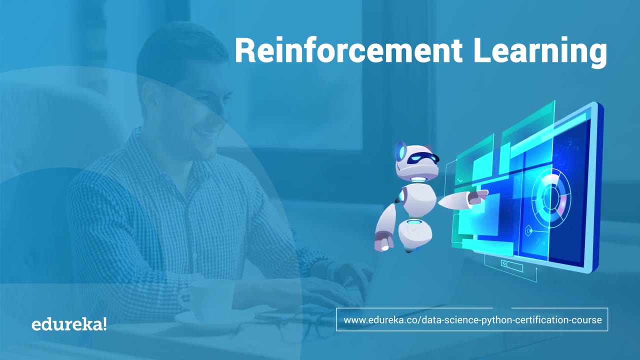 Good morning, good afternoon and good evening, guys, based on the time zones you all are coming from. So before we get started, let me quickly introduce myself to you all first, so you can be aware of the person you're talking to. So my name is Nidil Chakeria and I have been working in this IT. 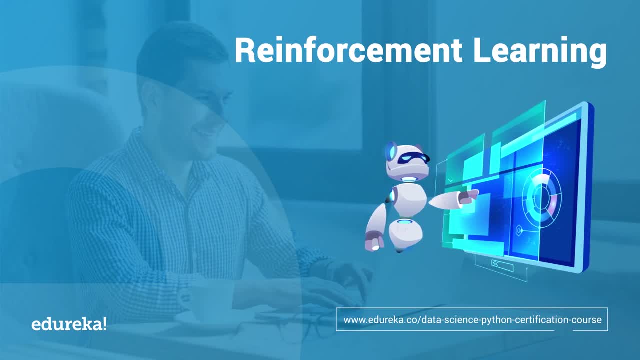 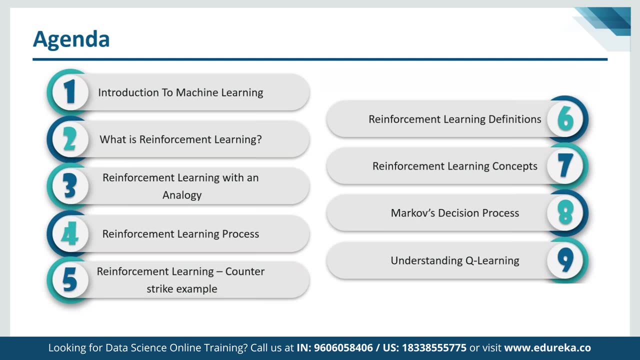 industry for more than 12 years now. So now let's get started. So the main agenda for today's session is: we are going to discuss on the introduction to machine learning, Then we are going to discuss on what exactly is reinforcement learning, Then we are going to understand. 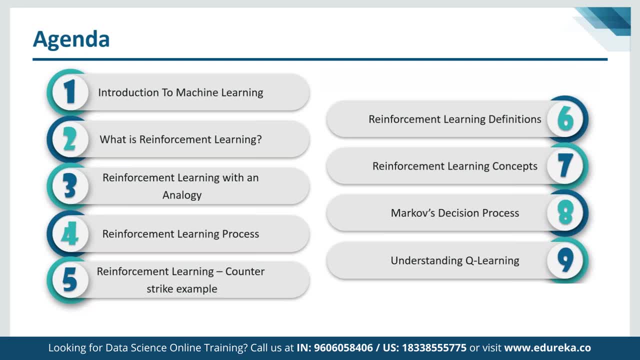 reinforcement learning by using a simple analogy, and then we are going to discuss on the reinforcement learning process, how exactly it works. Then we are going to discuss on the counter-strike example, on how it is useful, how reinforcement learning is useful in the popular game for. 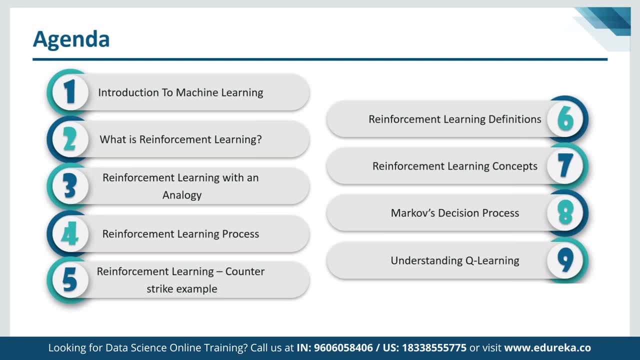 counter-strike. Then we are going to discuss on the component of reinforcement learning, different definitions. Then we are going to see the learning concepts. Markov decision process will be having an understanding of how the Q learning works. So that's the agenda that we 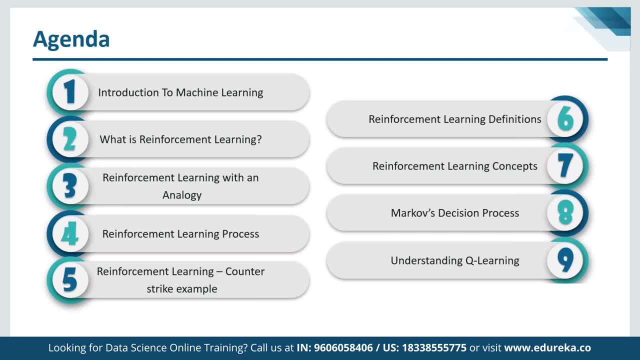 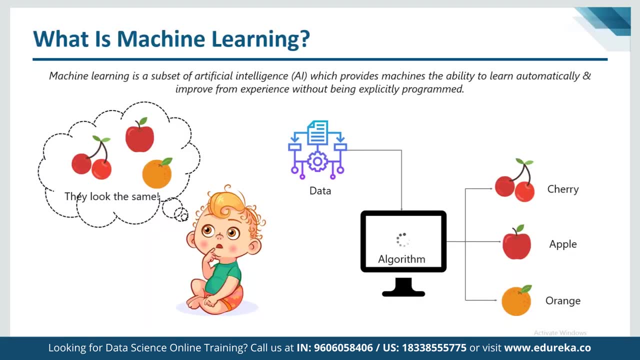 are going to cover as a part of this entire session today. Now, first of all, let's start with a discussion on machine learning. Now we know that artificial intelligence and machine learning, they all are among few domains, right? So there are most, we can say, the top trending. 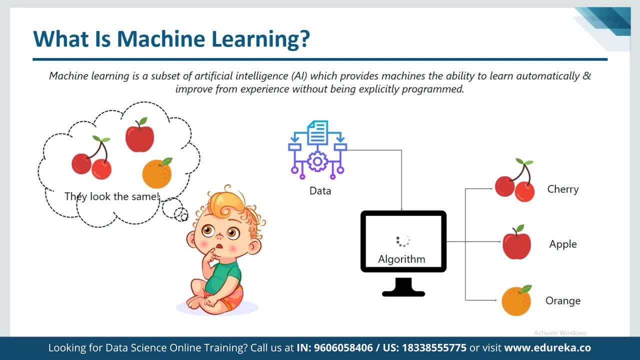 skill set, especially since last four years now, and we know that AI is going to create almost 2.3 million jobs by 2020, considering its main goal is to achieve machines to mimic human behavior. right So? because, again, artificial intelligence is nothing more than how exactly? 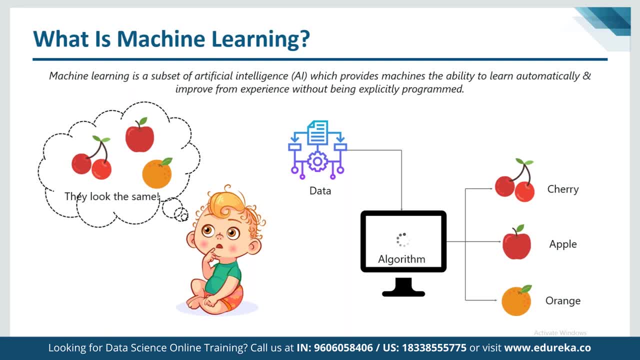 we train any kid- For example, when we are training a kid, okay, how exactly an apple looks like or how to differentiate between Apple, orange and cherries- and we have to first of all train the kid using the MMI, showcasing the kid the images and then labeling them, and then train and 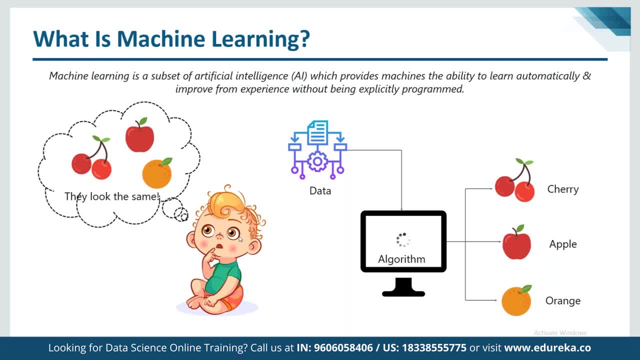 then multiple methods to which we can train the kid. So that's why we have first of all the machine learning concepts and then the machine learning is totally dependent on how much of data we are using for training a system. more data we use, more accurate. 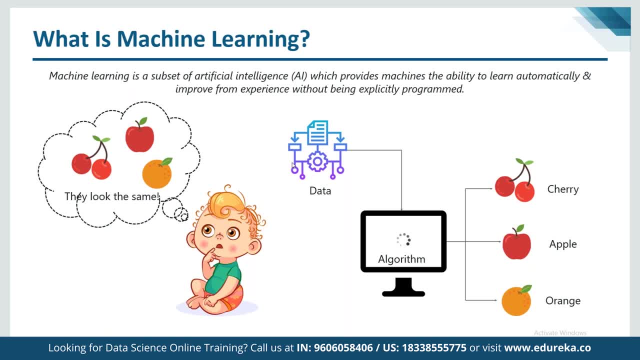 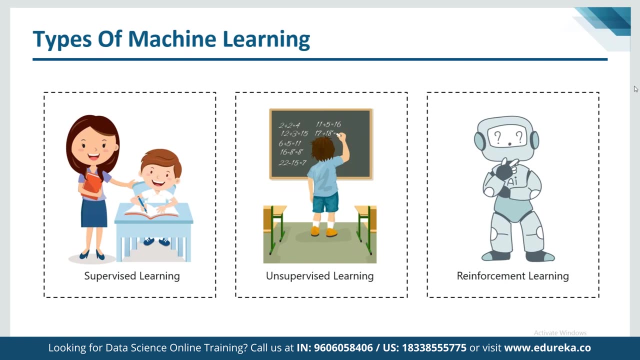 The results are going to be By combining whatever they have learned as a part of machine learning, then making a mind this with the algorithm to get these that results out of it as a part of machine learning itself, And basically there are three types of machine learning available that we have supervised. 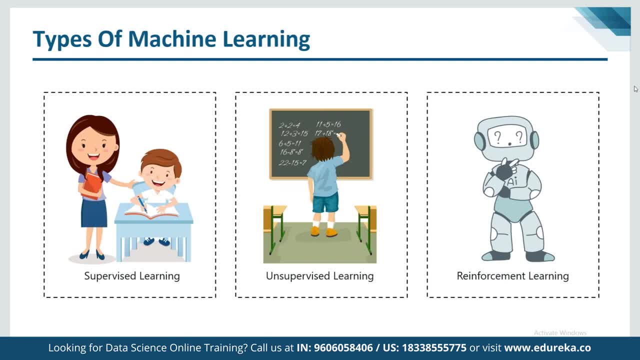 unsupervised and reinforcement learning. So when we say supervised learning, we simply train the system by giving a label data set. when it's a label data set, for example, we are training the kid now instead of just by showcasing these images here. 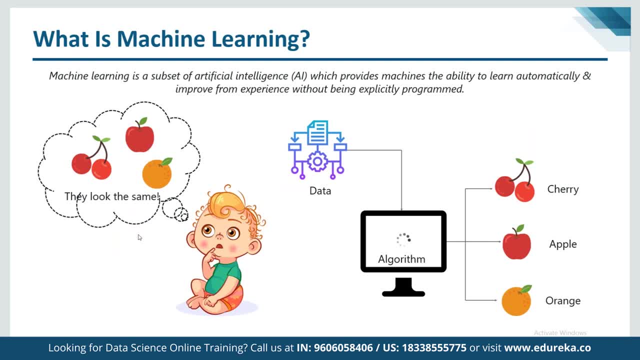 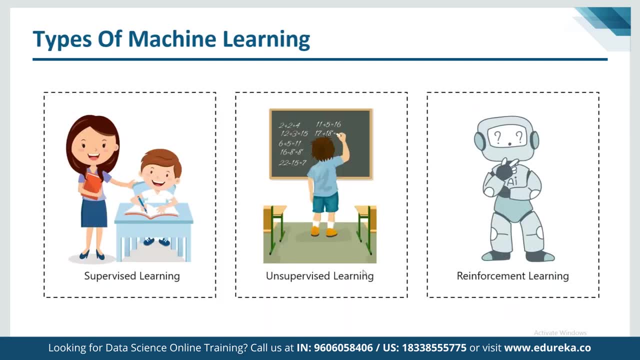 We can label care that this is Apple, This is orange and this is cherry, and then they can try to match the same pattern as a part of label data Correct. Same way when we are focusing on unsupervised learning, when we have trained the kid and 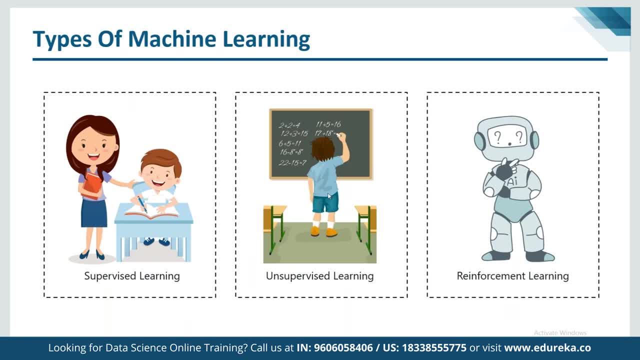 now we are letting the kid perform the action on its own right. So, for example, when we have free naked, okay how the addition works. now we can let the kid perform the addition on its own, especially when that is why we have unlabeled it as it. 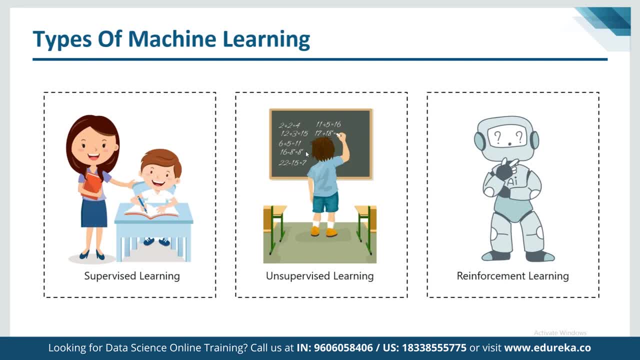 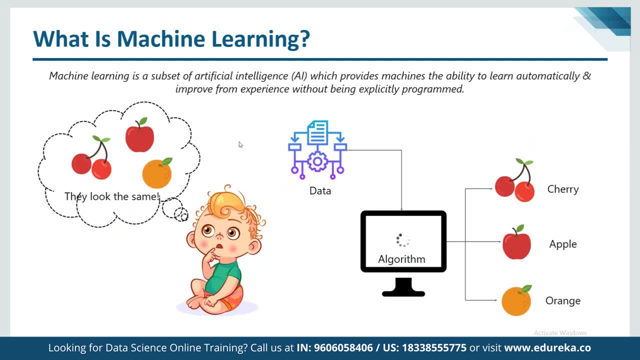 So in unsupervised learning, Okay, Okay, We mostly work with the unlabeled data set, so we can simply showcase the images here. For example, let's say we are focusing the images here and now we get them- images of banana, of of guava and again for other fruits- right, and then they can separate these three. 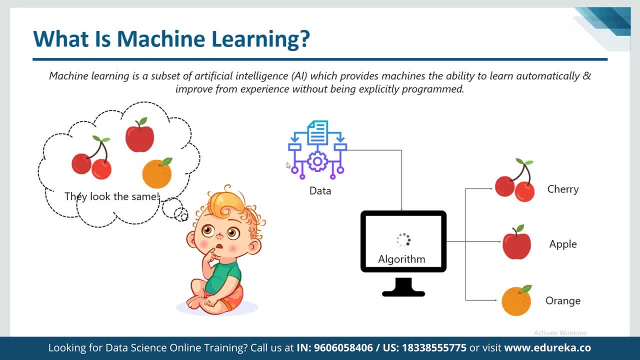 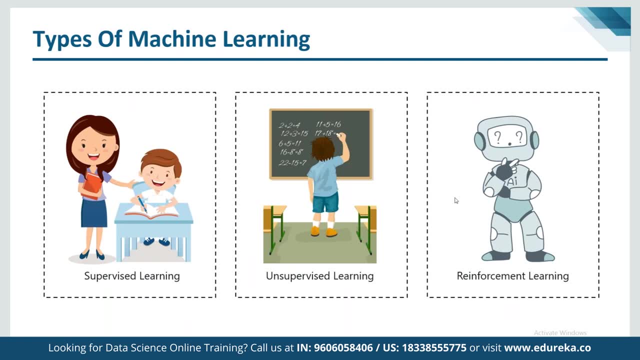 fruits from the other fruits as a part of, and they, even when we have the data sets, unlabeled as a part of unsupervised learning method. and then we have reinforcement learning. So reinforcement learning is basically Taking the input as a part of feedback, right? 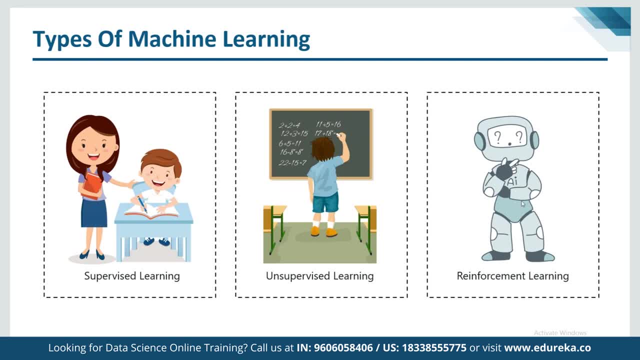 So basically, it's simply allowed, not, it's simply a. we can see a branch of machine learning that permits system to learn from the outcomes of its own decisions. For example, let's say we have treated system gate that okay. when done again, simply close the system by using control X right, as opposed if the system tried press, now use learning. 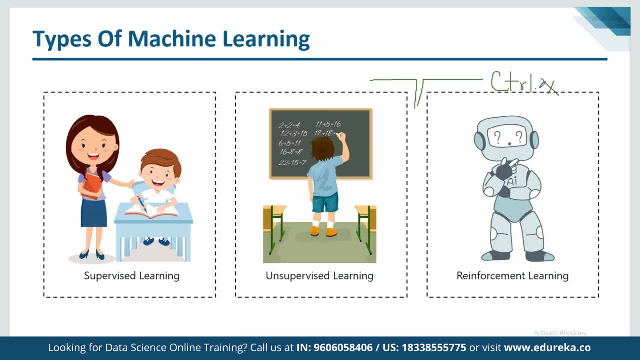 the command for control X and control X didn't work. instead of control X, control C works Correct. So now our system can correct its entire structure accordingly to that means: now this program does not work, Now it can go for the other variation as well. 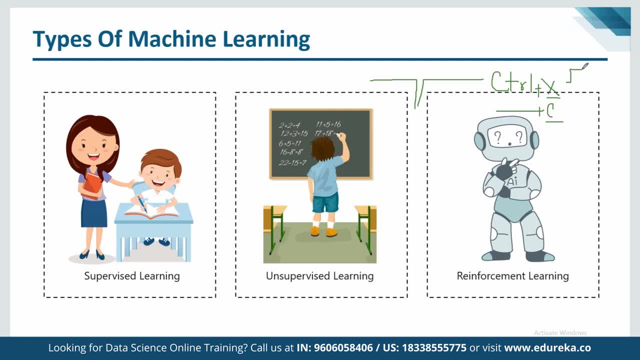 So, based on the feedback, okay, suppose, for example, whatever they have done is right or wrong, or suppose what is the output that has been generated. So, based on how well, based on the action they're performing, we can be allowing the system to learn from their own outcomes, right? 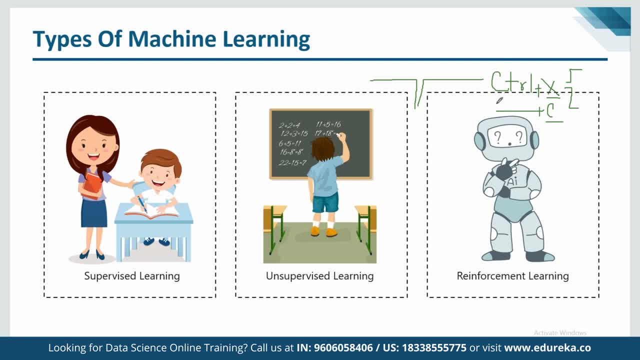 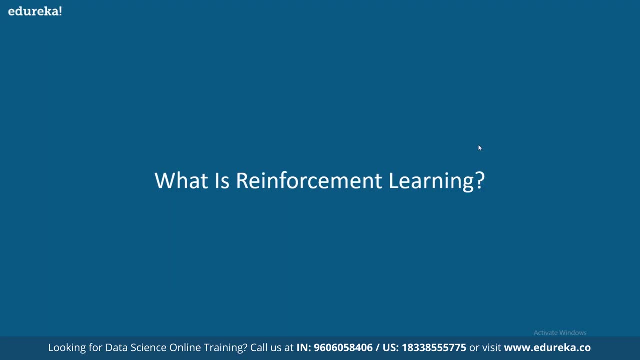 So that means we have a continuous feedback taken into account as a part of reinforcement learning models, And that's what these are three main machine learning models that we use in a real-time use cases. All right, and if we have to elaborate reinforcement learning, is reinforcement learning as we have. 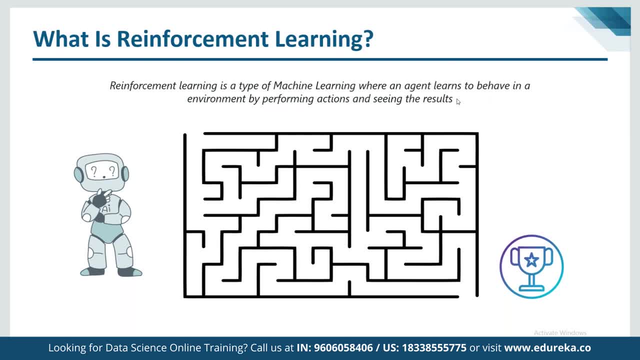 seen. It is basically a type of machine learning where an agent- or that means we can see a bot- learns to behave in environment by performing actions and seeing the results. for example, not if the board moves. starts to move here, right in the mark. moves here again, it sees. 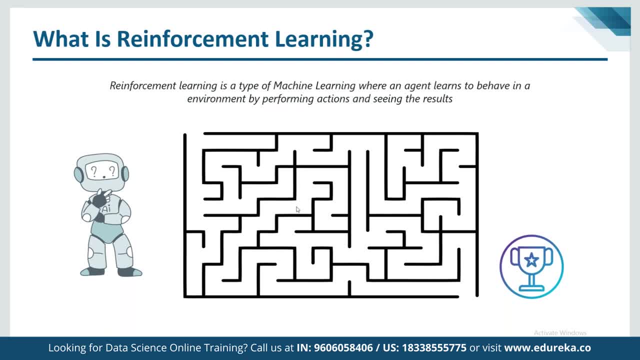 a closer. So whenever the bot observes a clothesline to, we can say in front of that board itself: and that board is not going to go forward in the same direction ever, correct? So that's why it is simply self-correcting its entire course based on the feedback. 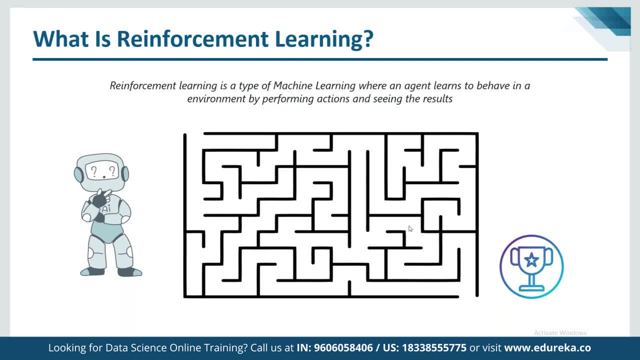 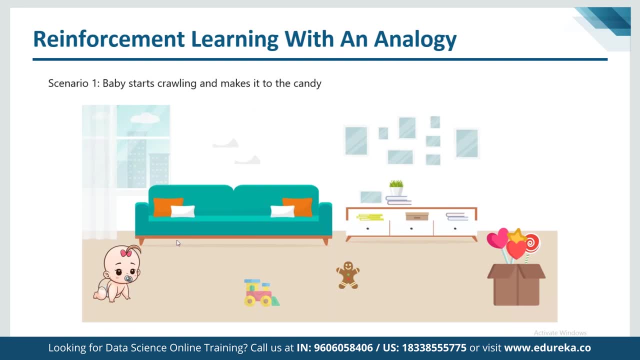 It is going to observe here and that's why this is going to simply rectify its own course in order to reach, we can say, complete- the entire goal itself. Let's understand with a simple example of baby. right Again, Here we can take the example for a baby to understand how the reinforcement learning. 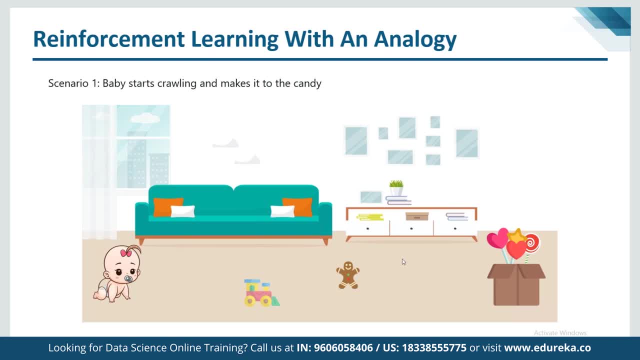 works. Now, let's say, baby starts crawling and make it to the candy. Now suppose not be a baby, start crawling here and again, without facing any kind of hurdles, the baby reach the candy itself. and now, when we double the way, when the baby starts crawling, 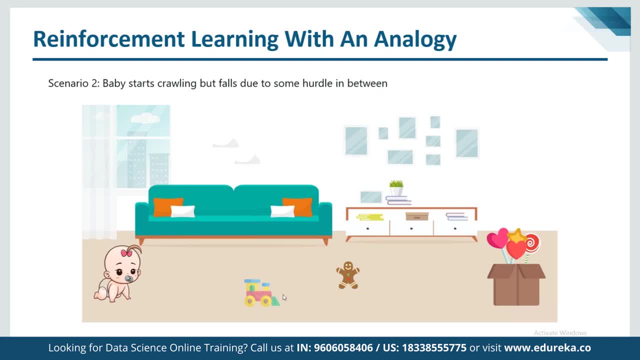 but fails to do some orders in between and the baby started crawling here. Now they may be certain hurdles, They may be multiple toys in between, like this one, and now the baby cannot proceed further Because Of the presence of this entire hurdle. correct, now the baby starts with, but not the baby. 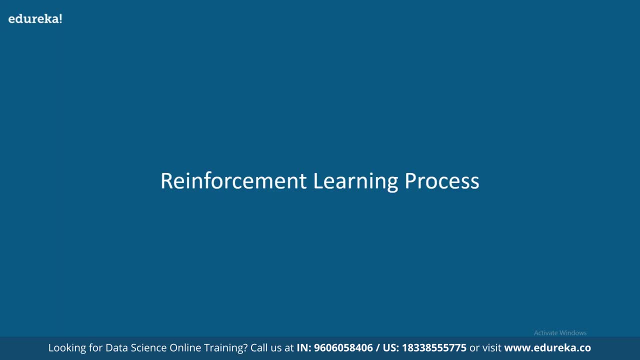 will simply take a pause for a while and again, then, if the baby has to learn how to overcome this hurdle and then how to remove the hurdles in order to reach to the goal that we have been designed for, and that's why they are two main core components as a part of reinforcement- 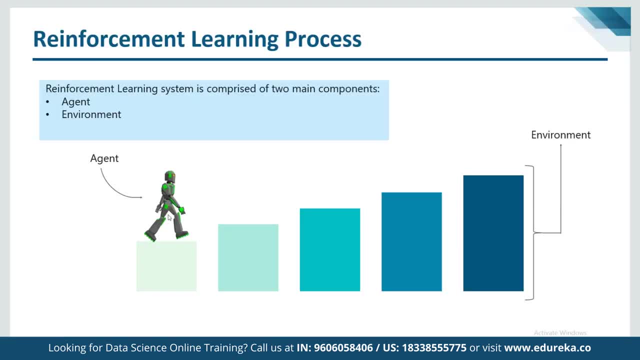 learning, We have agent and then we have environmental. agent is basically the part that is trying to automate the entire task. Correct, Whereas bought against. the environment is the factors, that is, that we have to take care of as a part of the learning process. 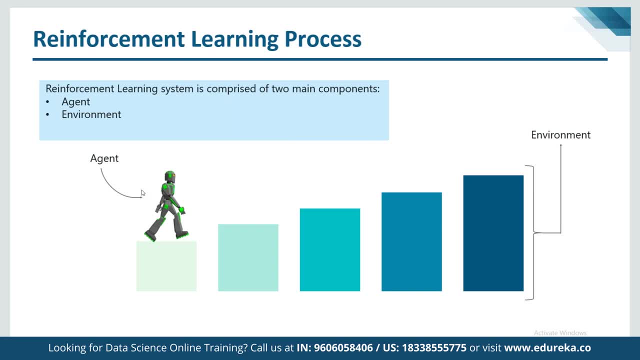 Right same way. now we can also take the example for any automobile factory as well. For example, let's say we are at an automobile factory filled with robots. Now these robots have the factory workers by conveying the necessary parts required to the assembly car. 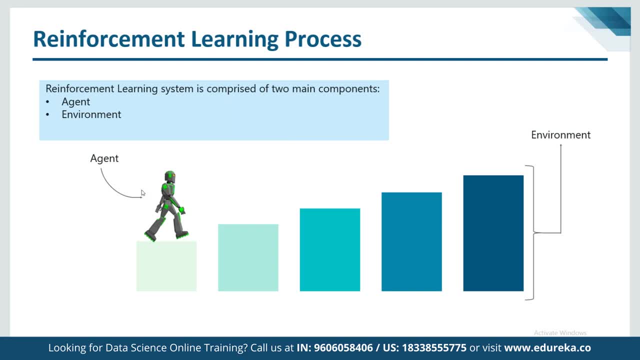 Now These are different parts That are located in different locations within the factory night stations and the parts now the parts can be Chess's wheels, dashboard, the music systems, the engine parts and so on, and the factory master has prioritized the location where Chess has been installed. 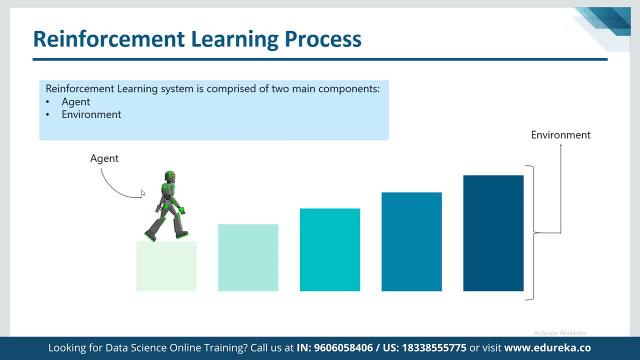 as the highest priority. And then we get now. the location at which a robot is present at a particular instance is called state, And that is at least what we are going to discuss. So we are going to discuss on the components of states actions. 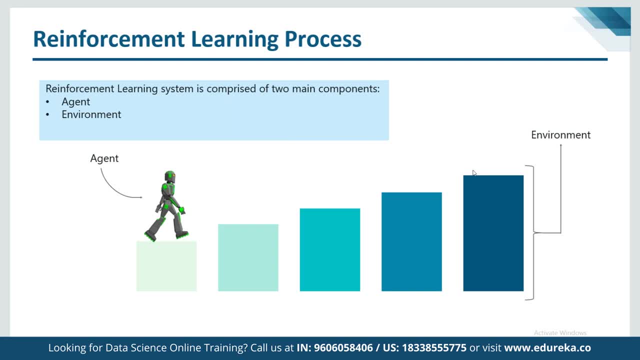 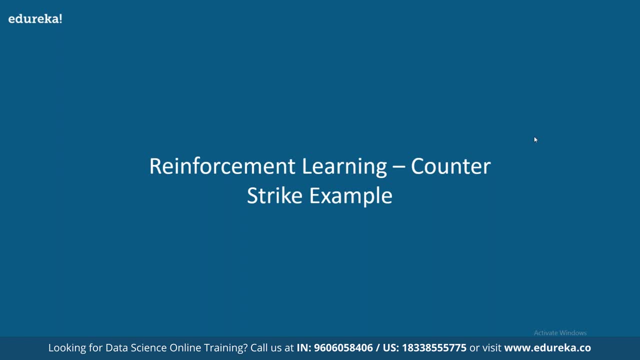 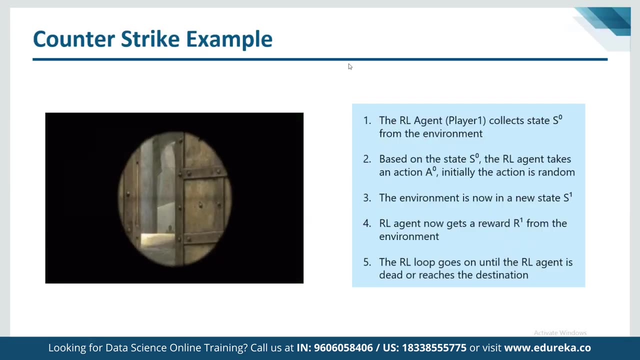 Rewards as a part of the question that we have to take care of when we are designing the reinforcement learning models. Now, based on the understanding for reinforcement learning, We can also apply it in a real-world scenario for counter-strike. So, for example, say now the RL agent, the player one, for example. 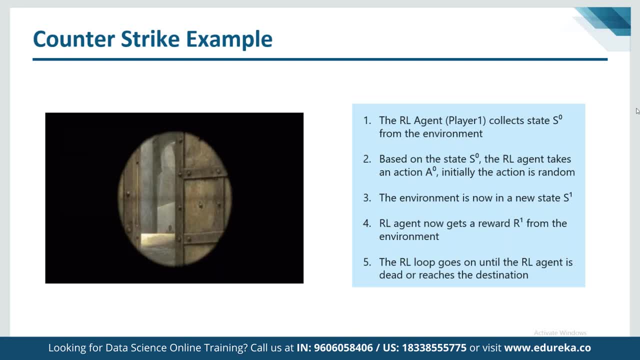 we have a player, one the player, one color state from the environment. the play. the main purpose of players are to collect the states right and then, based on the states the are in the RL agent, As in the player, takes an action- if we can refer to the action as a not- and then initially. 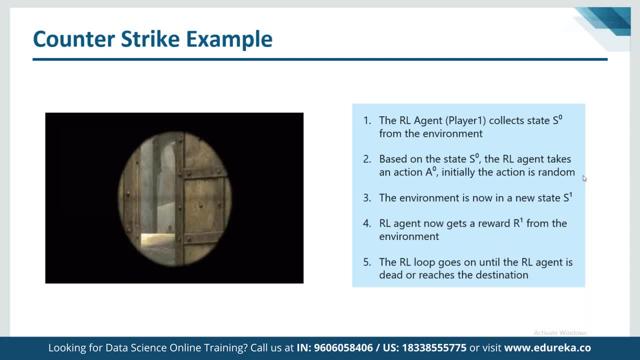 the action is random and now the environment is now in a new state and the agent, the players, now get a reward from the environment and the RL loops through the until the RL agent, that is, a player, is dead or it reaches the entire destination itself. So, based on the feedback received- or we can say feedback as a reward- then the same reward. 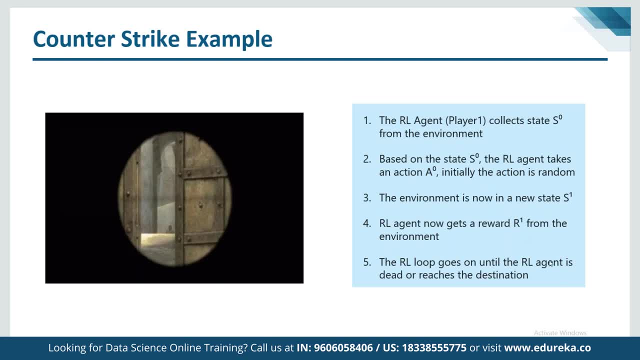 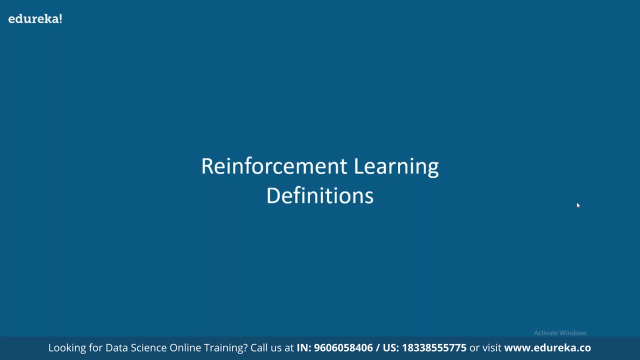 again, is taken into account. So, and that's why the entire agent, We'll go into loop until unless the agent is dead or it reaches the destination. So by taking into the consideration of multiple inputs. Now let's understand the basic concepts of reinforcement learning definitions one by one: 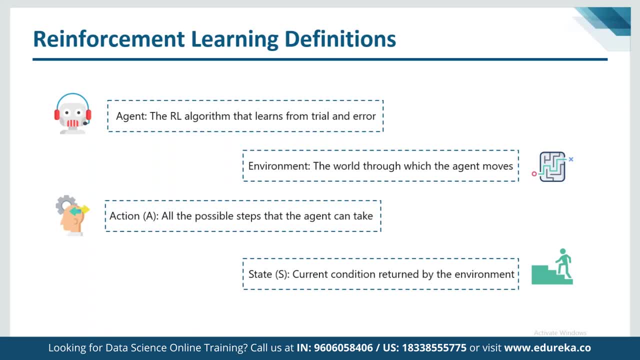 So first of all we have the component of agent, So agent is basically the RL. RL refers to reinforcement learning, So agent refers to the algorithm that learns from the trial and error. So basically it has multiple inputs and can start learning one by one right and then 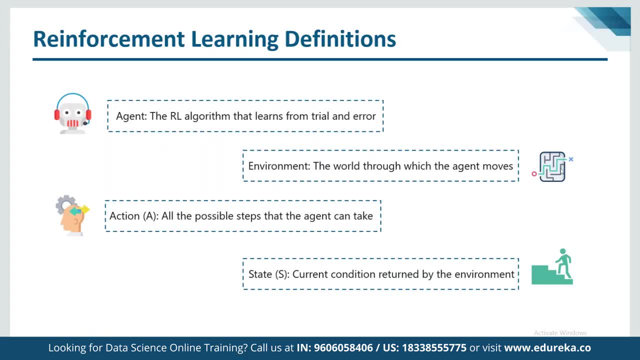 we have environment, So environment is a world through which the agent moves so that it can run the hit-and-trunt method. action is all possible steps that the agent can take, and stairs and state is the current condition returned by the environment so that that particular condition can be taken. 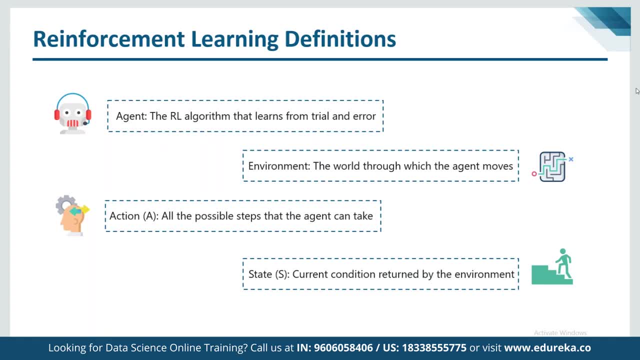 as a reward or as a feedback, and then it can be applied to modify the actions, So that particular condition can be taken as a reward or as a feedback, and then it can be applied to modify the actions based on whatever it has been given. then we have rewards. 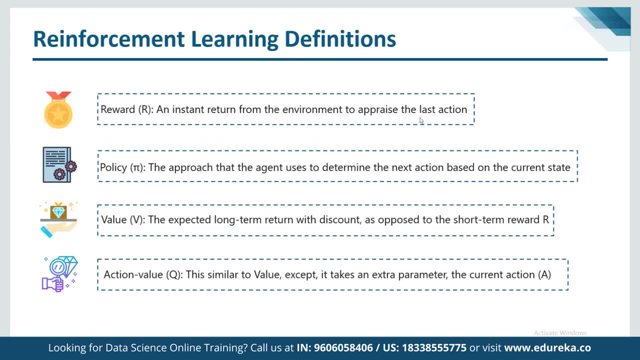 or reward is basically an instant return from the environment. to appraise the last action, We have policy defined by fire. So, again, the approach that the agent uses to determine the next action, based on the current state, And then we have value. So value is the expected long-term return with discount, as opposed to the short-term reward. 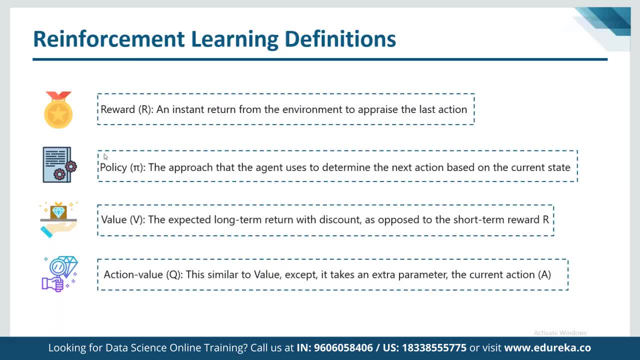 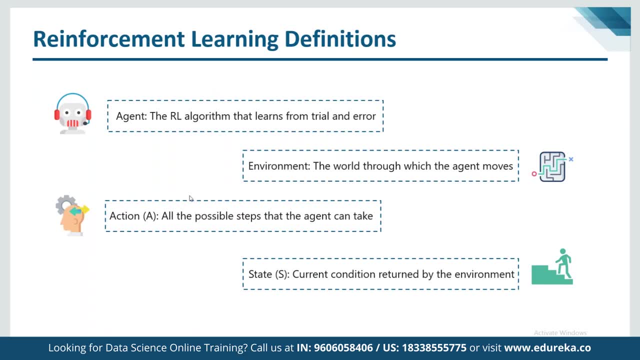 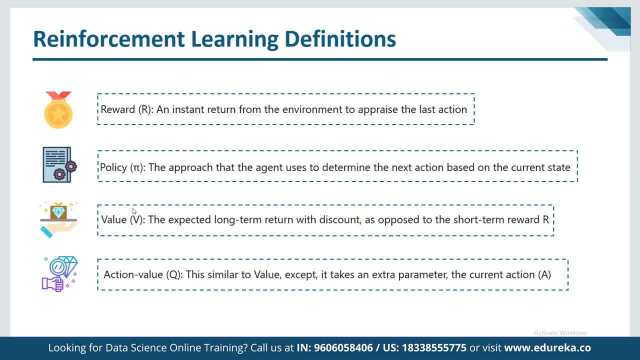 And then we have action value. So these are the multiple abbreviations that we are also going to use. so to have a quick recap, now we have agent, environment action state, then we have reward, the appraisal from the last action, then we are going to have policy, then we are going to have value, the 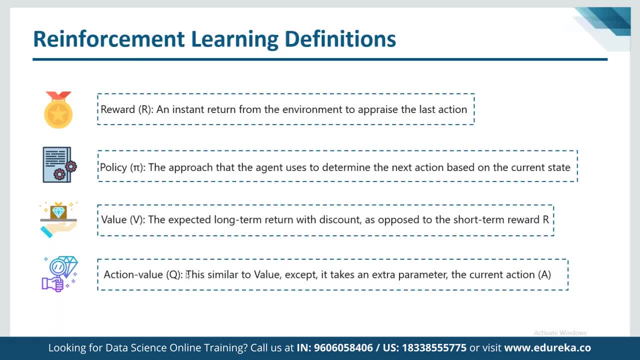 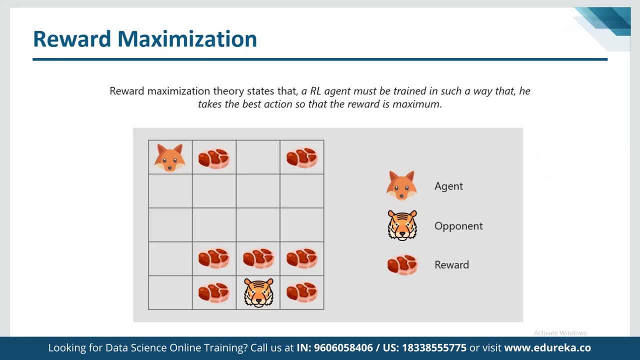 expected long-term return. and then we are going to have action, ask you, similar to the value, except it takes an extra parameter, and the current action to be a lesson sign on the reinforcement learning Concepts. So, in or not, reward maximization Theory states that an RL agent must be trained in such a way that 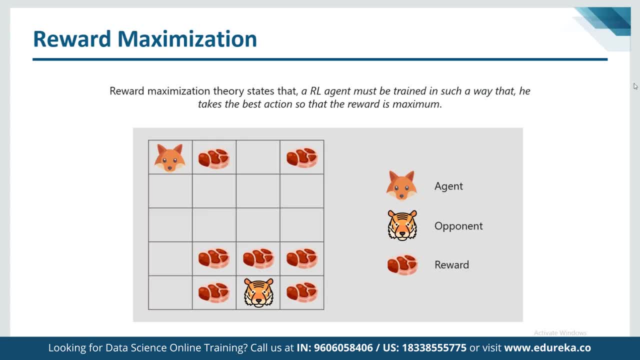 he takes, he or she takes the best action, so that reward is maximum right. So with minimum number of steps required, here, the reward should be maximum. That's exactly is how the entire structure is defined here in terms of reinforcement learning example: here We have agent, then we have the opponent and then we have the 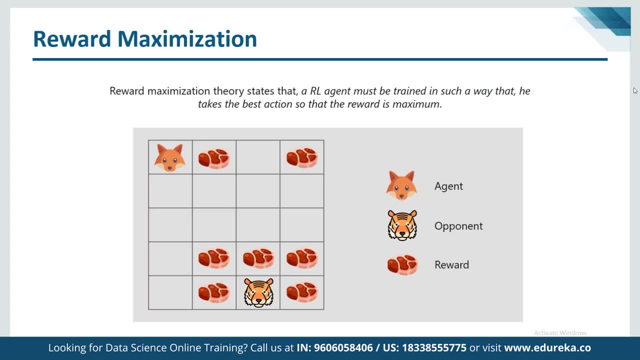 reward, so that we have to take it and they have to take the necessary steps in order to get the maximum output of any given learning. and then we have the component of exploitation is. it is basically about using the already known exploited information to hide in the reports. 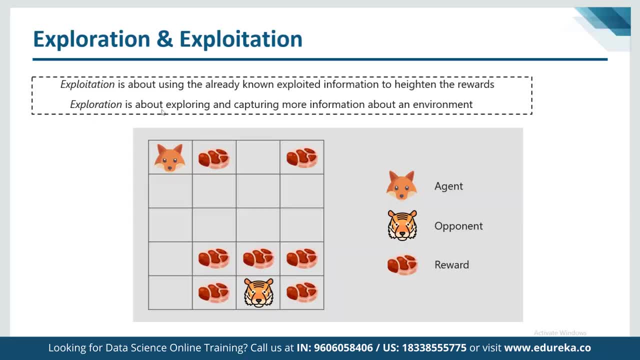 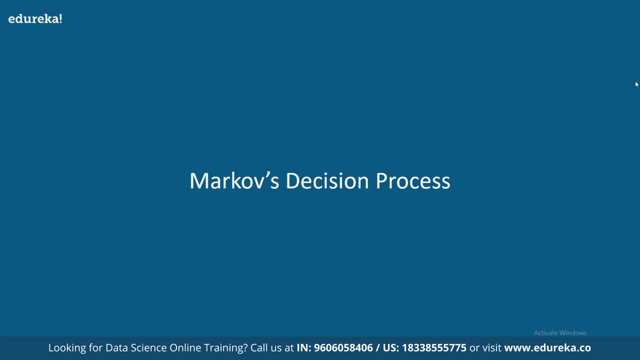 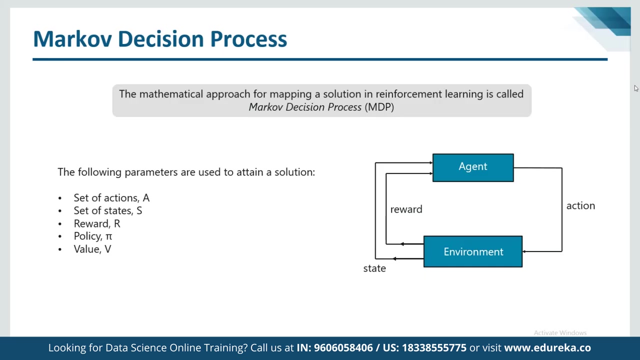 That means going for what exactly works, and exploration is about exploring and capturing more information about environment, something which has not been tested yet, and then we can go for hidden trial method. Let's also understand on the components of Markov's decision process. So basically we can say Markov's decision process is basically a mathematical approach. 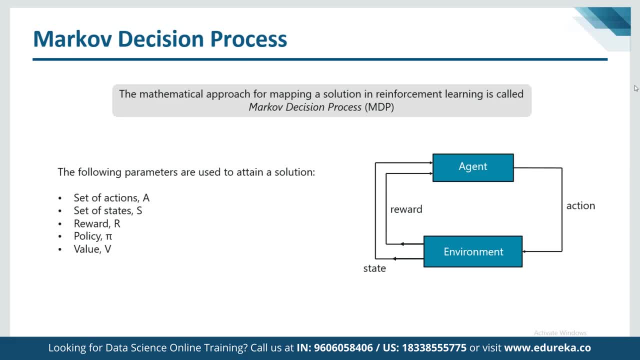 I can say it's simply a process which is a discrete times- We can say time control process. It provides a mathematical framework for modeling decision. It simply provides a mathematical model to frame the model- We can say that the decision-making process- and where we can use it for situations where 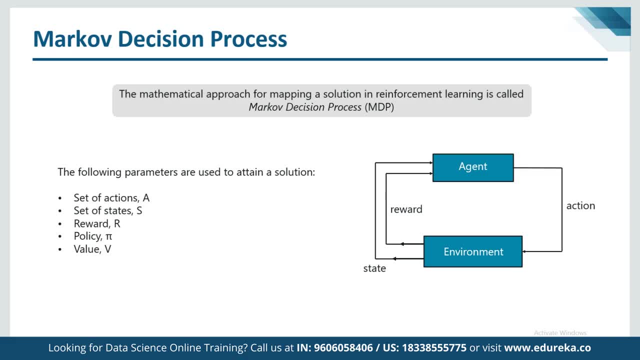 outcomes are partly random and partly under the control of a decision maker. That is actually is what Markov decision is all about. So basically, it's a discrete time control process which is basically useful for providing a framework for creating the models in situations where outcomes are partly random and partly under the control of any decision maker. 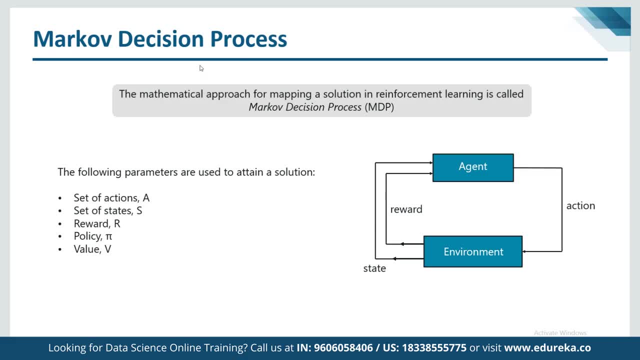 That is that he is what Markov decision process is all about. These are the following parameters used to attain a solution that we have: set of actions, a set of states, rewards, policies and value. These are all the factors that we take into account when we are working on Markov decision process. 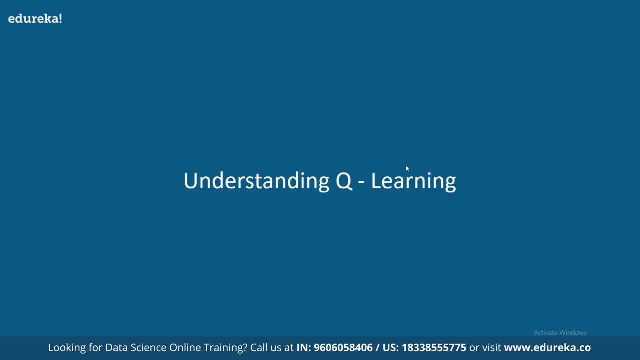 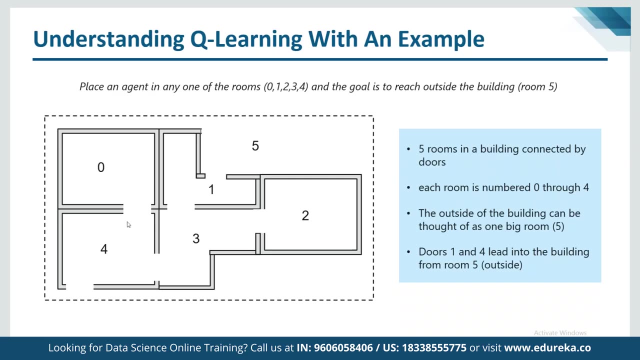 Now let us understand quickly on the components of Q learning. Now, when we are placing any agent in any of the rooms, for example, suppose we are talking about counter-strike, right? So we, when we are placing the agent- agent as in play- in any of the rooms, 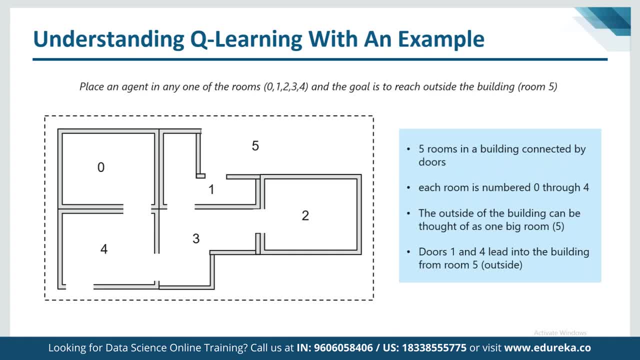 he has a 0, 1, 2, 3 for the goal is to reach outside the building That is room 5, now 5 rooms in a building, connected by those, and each room is numbered 0, 2 through 4, and the outside building can be seen. 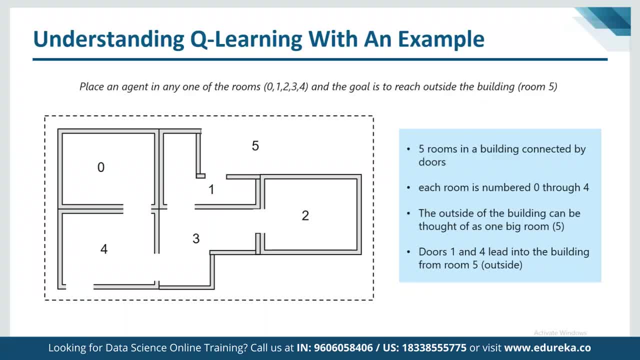 as a big room, as 5 and those 1 and 4. they lead into the building from room 5.. That is the from the outside. So there's only only two entries available inside this given parameter, That's, that is a door from room 1 and do from room 4.. 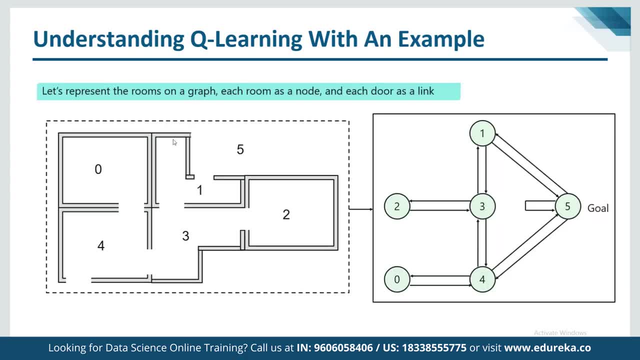 And let's represent this entire room on a graph and each room as a node. So we have second, we have third, we have for now. This is an inverted copy. So we have second room, then we have third, so we can come back and forth from second and third. then third is connected to room 1, third. 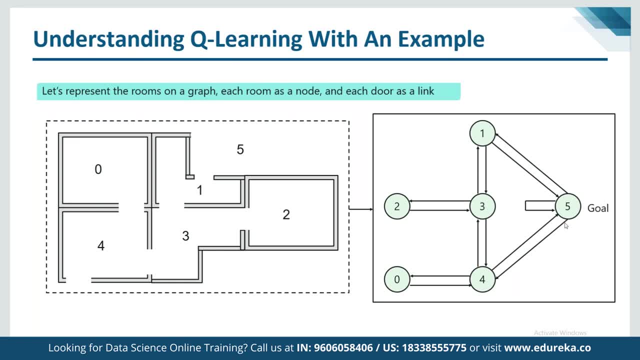 is also connected to room 4 and the main goal is to reach room number 5 and for reaching through room of 5.. We have to go through the door 1 and door 4 because these are only two exits to the outer world, or we can say to the room 5 itself. 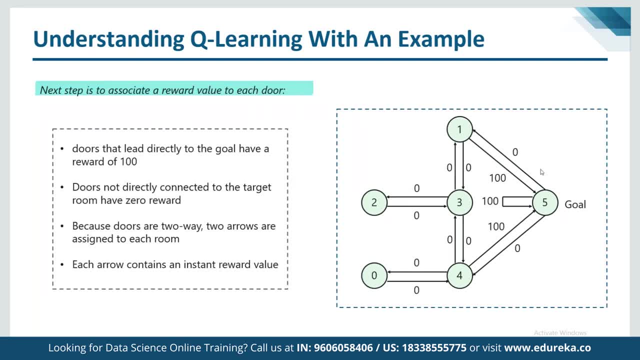 Now next step is that door leads directly to the goal have a reward of 100 because, again, the door that leads to the goal, or we can say door number 1 and door number 4. They will have a reward 100.. That means if the user exists from second to 3, reward is 0. 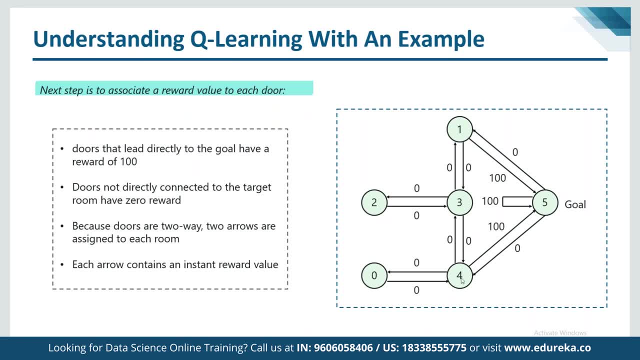 if the user exits 3 to 4, reward is 0. if the users come back from 4 to 3 again, reward is going to be 0. Same with the rewards for any other rooms are going to be 0, except if the user exists from room number 1 to 5,. 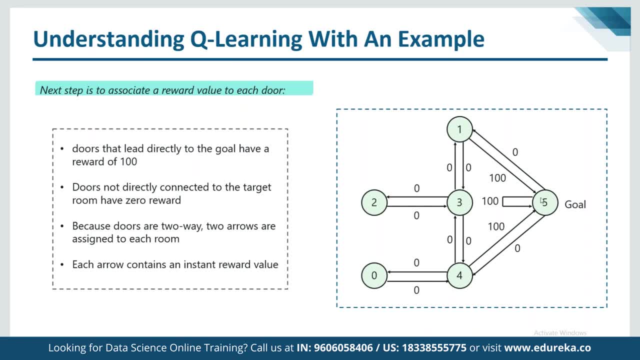 then the reward is going to be 100. if the user has landed into 5, but again it has not returned, then the reward is also going to be 100. if the user has exited from room number 4 to 5, then also the reward is going to be 100. right and exactly is how we can attach the reward value. 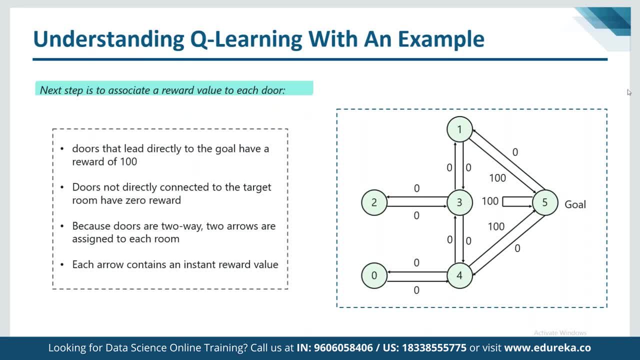 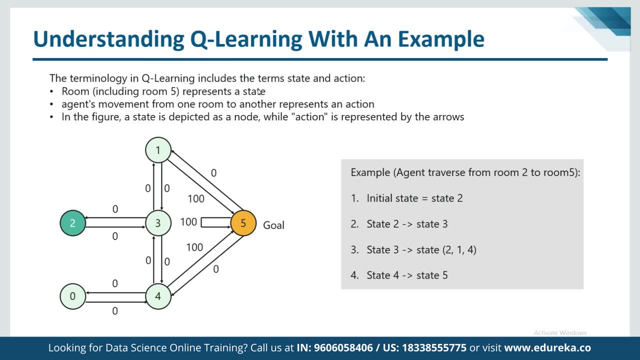 as a part of the entire reward parameters And the terminology in Q-learning includes the term states and action. So room including room number 5 represents a complete state. So obviously, suppose if the user comes from room number 2 to 3, obviously the state is going to be changed. 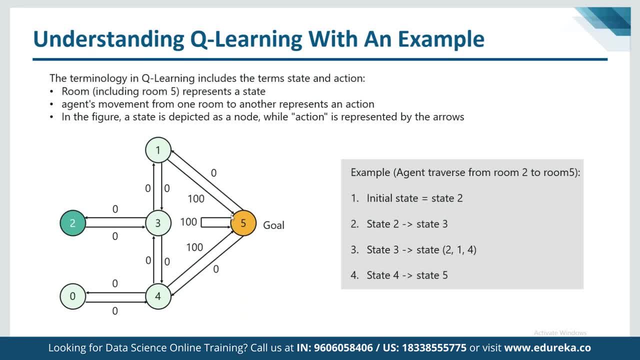 Same way from 3 to 1, 1 to 5. the states are going to be changed and agents movement from one room to the other is called an action. Okay, and in the figure the state is depicted as a node, while the action is represented by the rows. 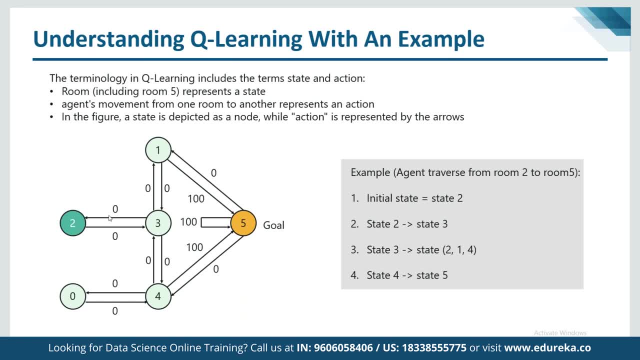 That means if the user comes from 2 to 3, then the movement here will be termed as an action, and when it comes to 3, then this current state is 3 and the action has been what has been performed. correct. That means initial state was 2.. 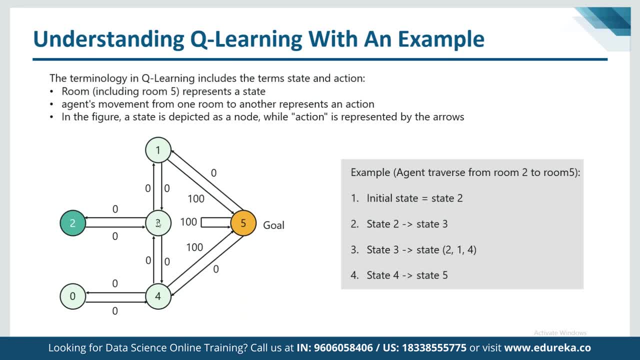 Now state 2 has been changed to state 3. here and from state 3 we have a possibility of going to state 2 again, state 3 or state. we can say state 1 or state 4.. There are three possibilities. and from state 4, 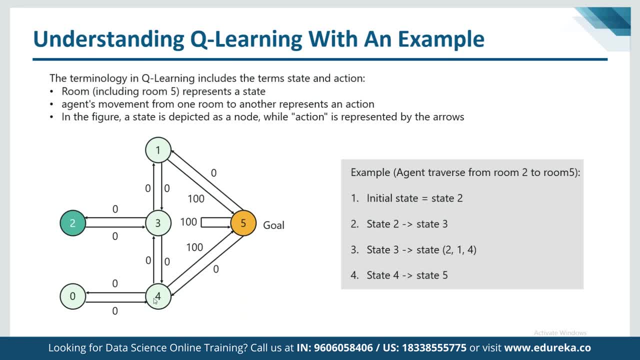 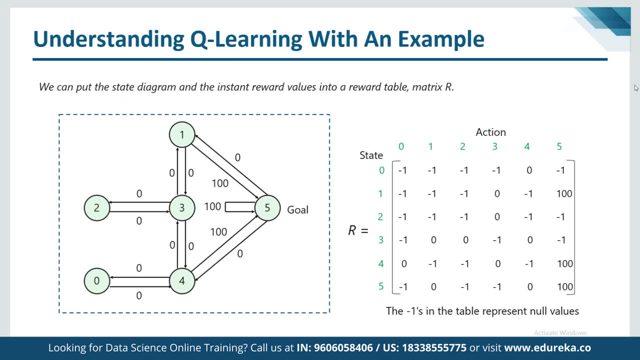 they are again. the user has gone from state 4 to state 5.. As a part of Q learning scenarios, and if we have to put this in a state diagram, then the- instead of what values- into reward table, then we can create the entire metrics here as an action as 0, 1, 2, 3, 4, 5. 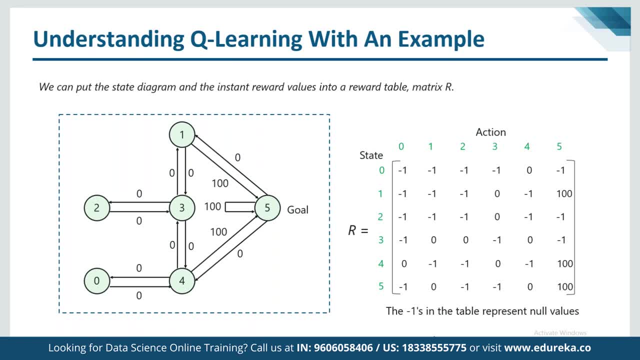 and then we have multiple states here And the minus 1 in the table represents the null value. That means from 0 to 0. if you go to 0 to 1, again no value. that means if you go from 0 to 3. here again, 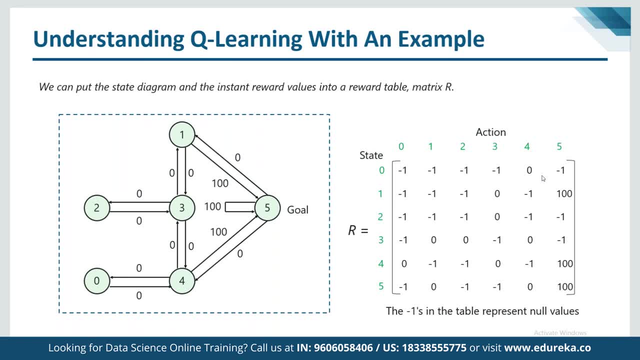 no value is 0 to 4 no value. But again, if you go for 0 to 5, because again we can't go there directly, That's why it is also having null value- But if you go from 1 to 5 only, then we are getting 100. 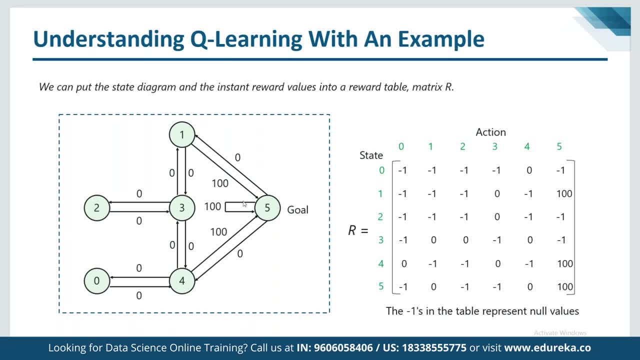 if you go from from 4 to 5, then we are getting 100, and if you remain in 5 itself, then only we are getting 100 as a part of null value. And when you say it minus 1 here, because again, 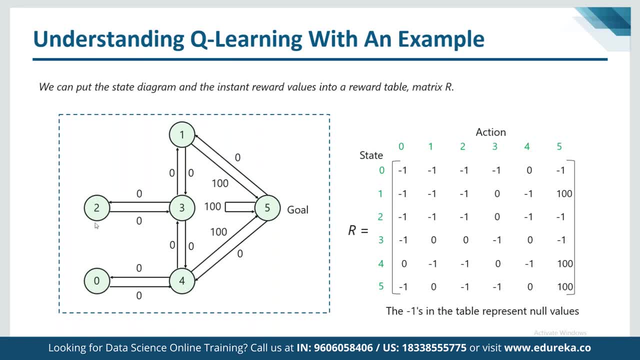 we know that 0. we cannot go from 0 to 1, 0 to 2 directly, right? That's why we have the value as minus 1, because there's no way, there's no interconnection between 0 and 2. we, in order to go to room number 2 from 0. 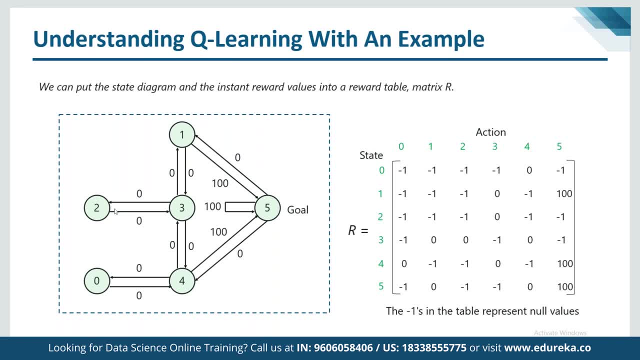 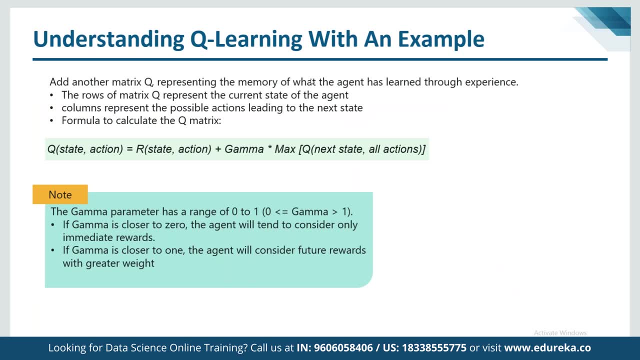 we have to first of all go to room number 4, then do number 3 and then so on, and that's how we had designed the entire matrix here. Now, next is we can add another matrix Q, representing the memory of what the agent has learned through the experience. 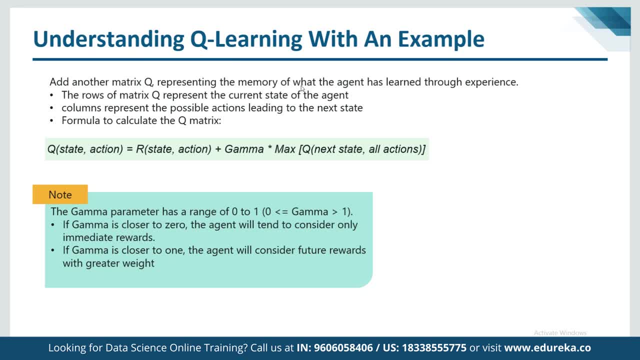 The rows of matrix. Q represents the current state of the agent, where, as the columns represent the possible actions leading to the next state and formula to calculate the Q matrix. We have Q, where we have state and action are state and action for the agent, and then we have gamma multiplied by Max for the same. 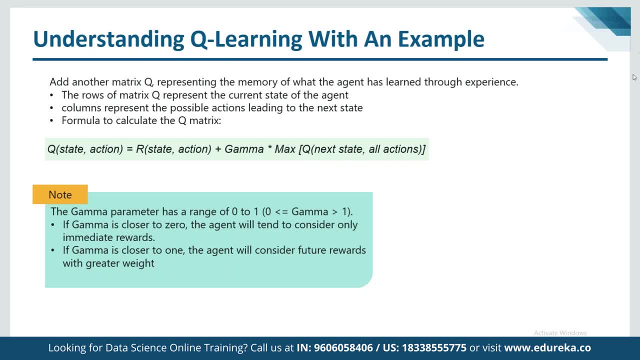 and the matrix Q, which is for next state and all the actions, and here the gamma parameter has a range of 0 to 1, where gamma is less than 0 and we can say a value between 0 and 1 itself, and if the gamma is close to 0, the agent will tend to consider. 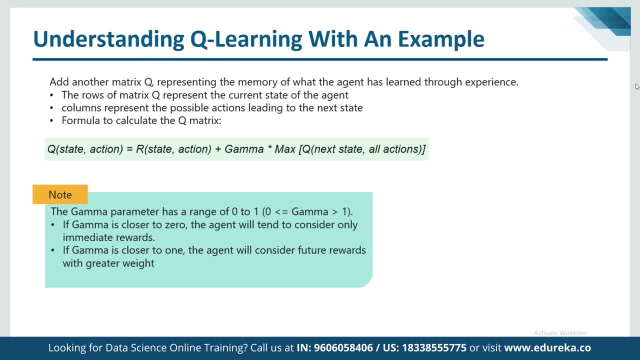 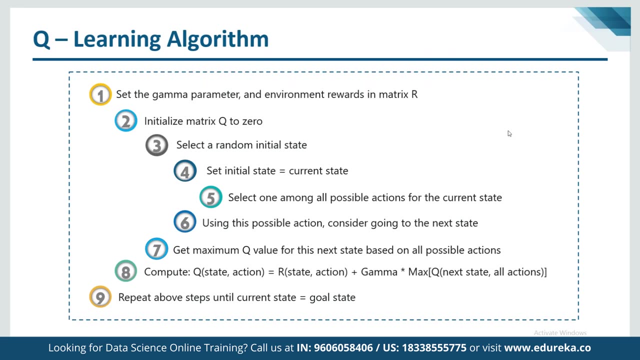 only immediate rewards, whereas if gamma value is closer to 1, the agent will consider future rewards with greater weight as a part of Q learning. And that's how. first of all, we have to set the entire gamma parameter and the environment rewards in metrics are. then we can initialize. 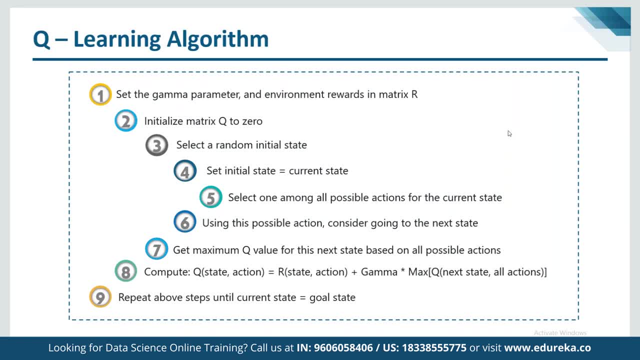 matrix Q to 0. select a random initial state. set initial state is equal to current state. select one among all the possible actions for the current state and, using this possible action, We can consider going to the next state where we can get the maximum Q value for this next state, based on all possible actions. 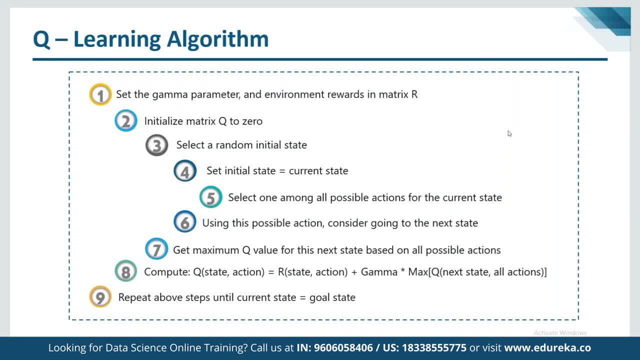 and then we have to find the computation by simply to find the Q state action, our state action plus gamma multiplied by Max for next state and all actions, And once all the steps are repeated then we can achieve the gold state towards the end, Putting this up as a part of metrics here. 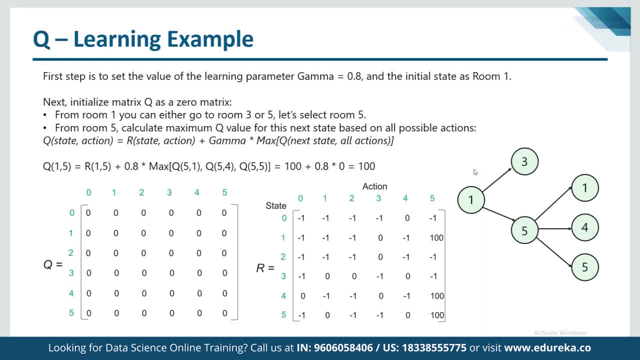 We can see. the first step is to set the value of learning parameter gamma, 0.8, and the initial state as room 1, and then we can initialize metrics Q as 0.. Metrics where, from room 1, we can either go to room 3. 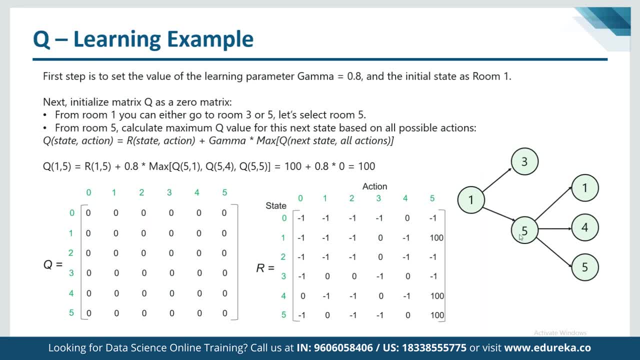 or we can go to room 5 and let's select room 5 here and from room 5 we can calculate the maximum Q value for this next state based on all possible actions. It's like we have Q state action and we have our state action plus gamma multiplied. 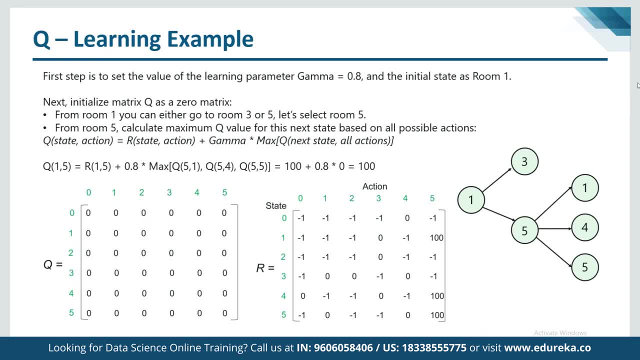 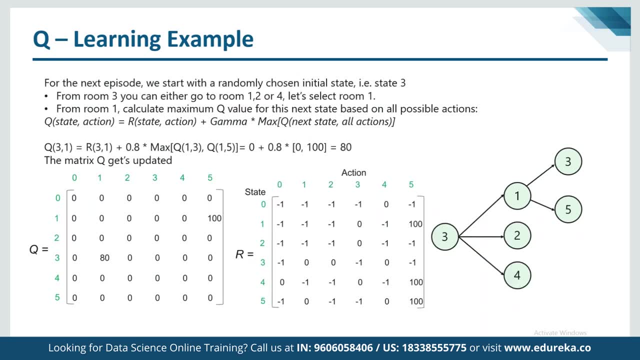 by Max as a next state and all the actions defined gamma value in is between 0 and 1 itself, And that's where, for the next episode, We can start with the randomly chosen initial set, that is 3, and then from room 3 we can either go to room 1 or 2 or 4. 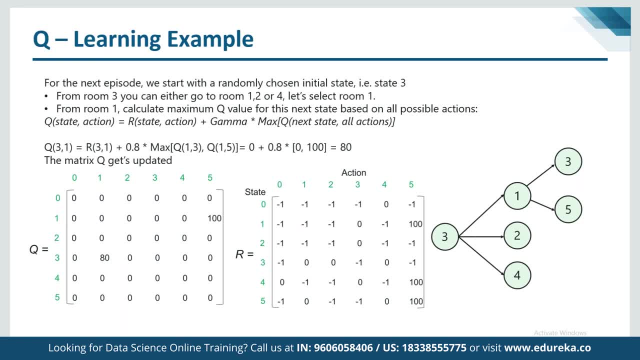 and here we can select room 1 and from room 1.. We can calculate the maximum Q value for the next state based on all possible actions where we can define Q a state action, state action gamma for next state, and all actions where we can start by Q 3: 1, because we are starting from 3 itself, and then 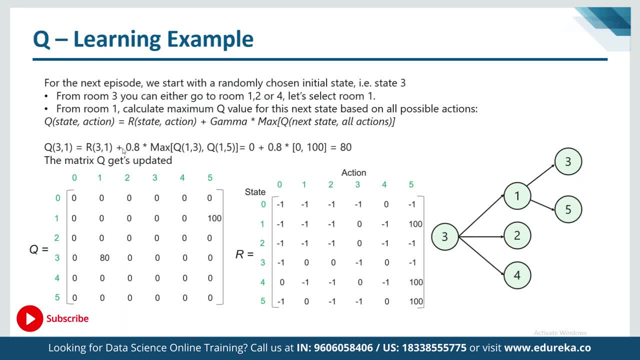 they're using the gamma value as your 0.8 multiplied by all the possible values of the initial value for the 3 and the gamma value from Q 1, 1 to 5, and it's how we can get the entire metrics updated. 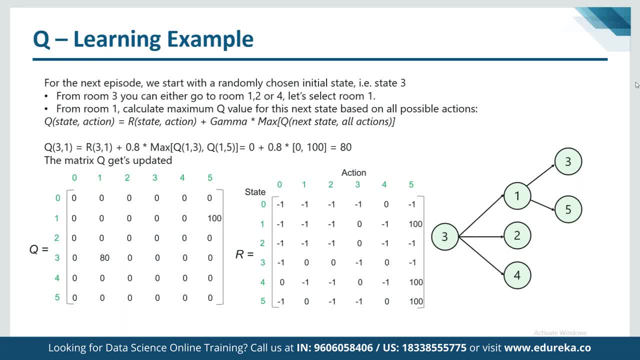 Are is simply the metrics that we are referring to, and again as a part of the continuation here, we can again start with the next state, for 5 as well, right, and then we can start from 1, and now, in the next state, 1 now becomes the current state, and then we can repeat the inner. 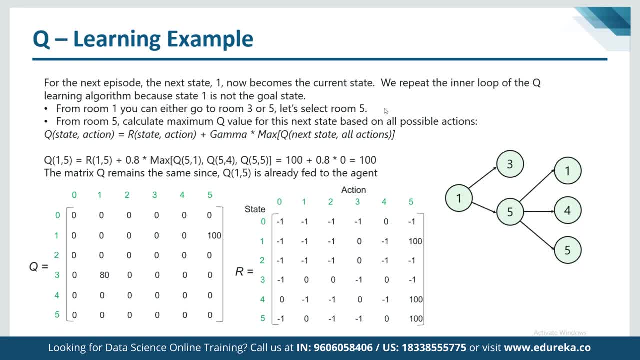 loop of Q learning algorithm. because state 1 is not the goal state, because state 5 is the goal state, right? So here we can. from room 1, we can either go to room 3 or 5, where we can select room 5, and from room 5 we can calculate. 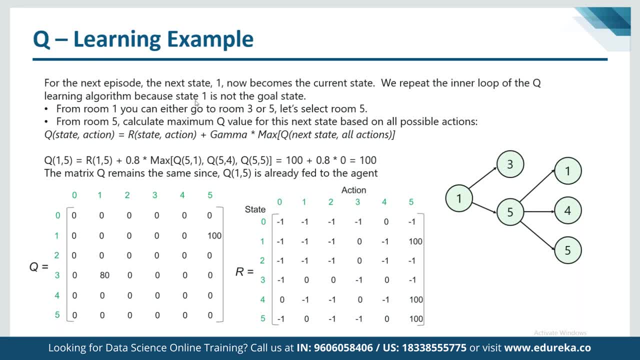 the maximum Q value for this next state, based on all possible actions, where you can find the Q starting point from 1 to 5 and then we can take the same gamma value to be 0.8 multiplied by 5, is to work from 5: 1, then 5- 4 and then from 5: 5..